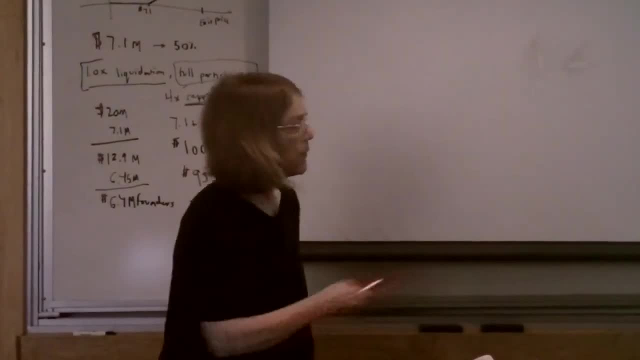 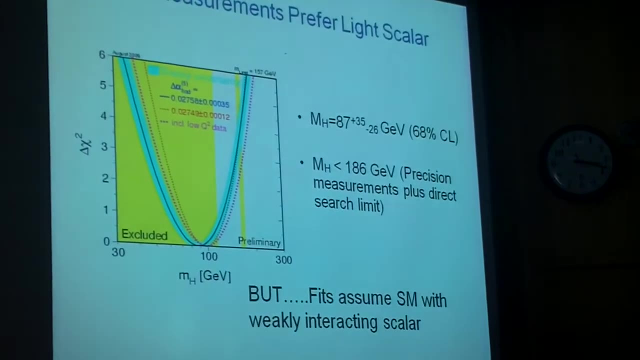 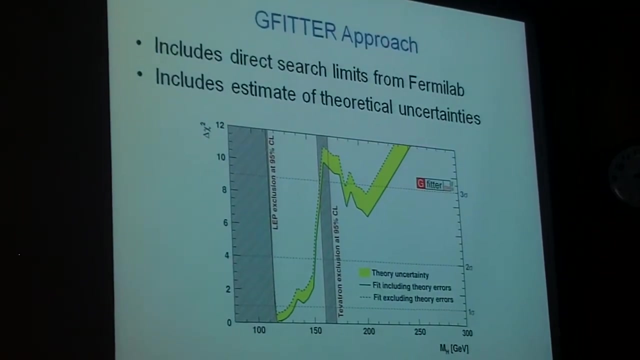 mind to prefer any point in this plane. here, However, these fits are indirect. They assume the standard model with the weakly interacting scalar, this minimal model, And it's, you know, a little bit of an error. Okay, So there's been another set of people who are 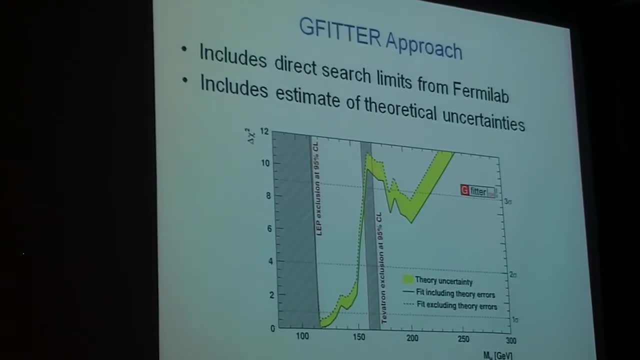 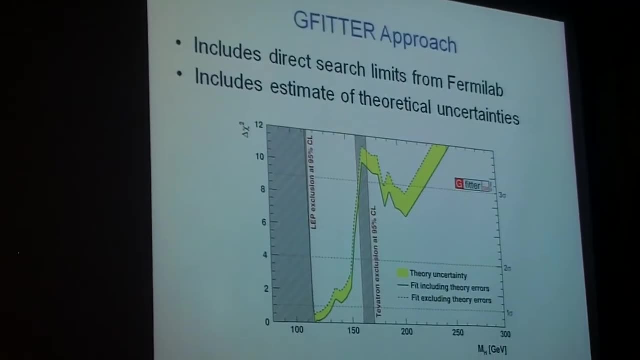 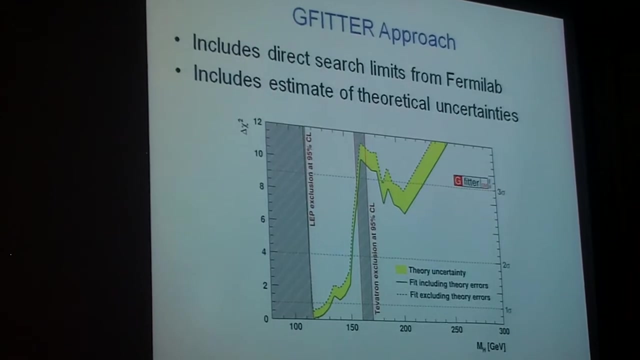 doing fits to all this data. This fit here is from the LEP electroweak working group. The GFITTER group is the group that brought you SFIT or CKMFIT, or they do a lot of fits to data, And so this is an independent approach. It's a chi-squared fit as a function of the 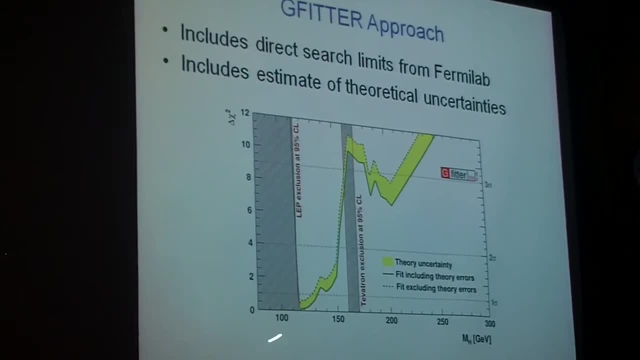 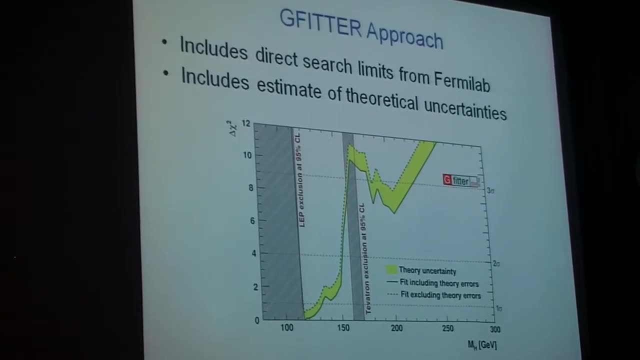 scalar mass, And this yellow curve here looks pretty much like the curve on the previous page. So what they have done is they've included direct search limits, which we'll hear about at the end of the afternoon. They've included those limits in their fit, And that's what. 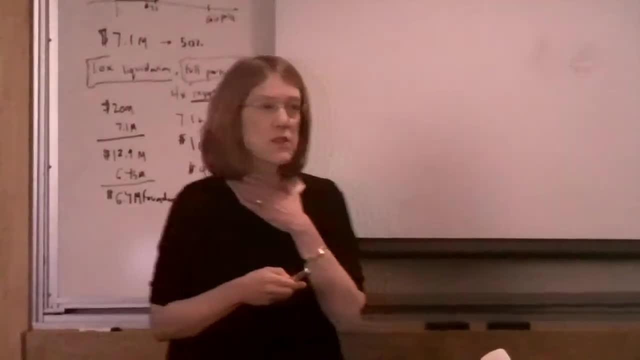 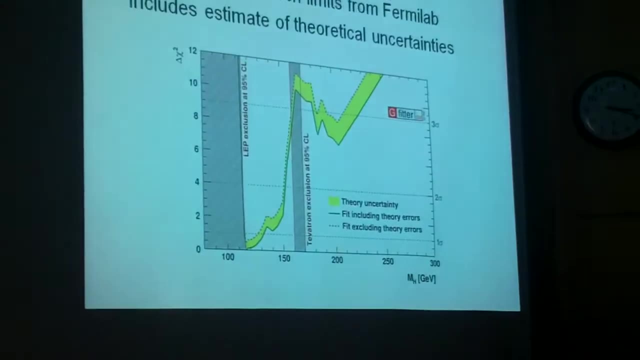 makes this kind of jagged here. So you can see that the limits from Fermilab are actually changing these indirect limits. The other thing they've done is they've included theoretical uncertainties, And you can see that there's a band on this, But nonetheless, the bottom. 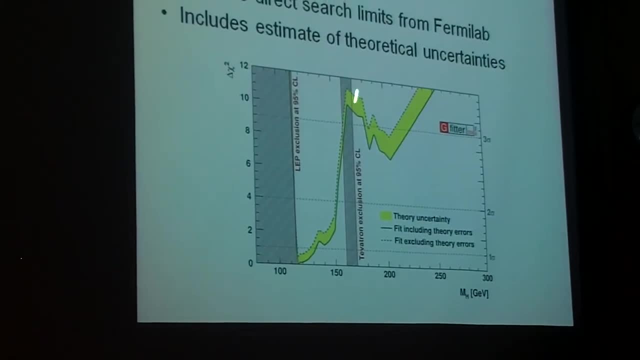 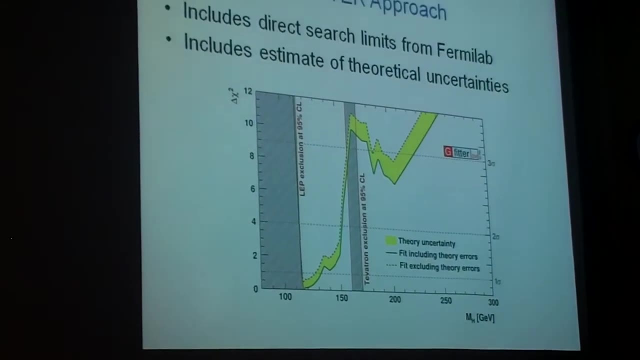 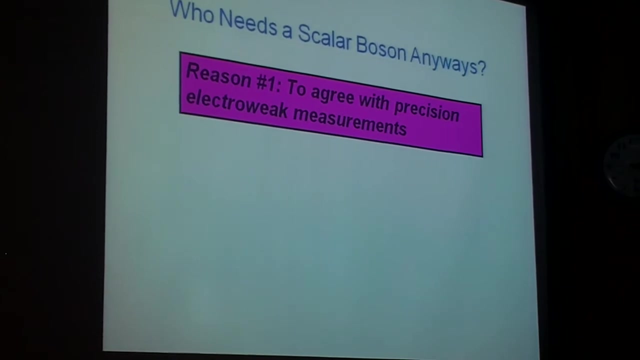 line is: here's the three sigma limit right here And it's about 160, 170.. So we expect that, if the minimal standard model with a single scalar is true, that this scalar is relatively light. So, in my pragmatic approach, who needs this scalar boson? Well, you need. 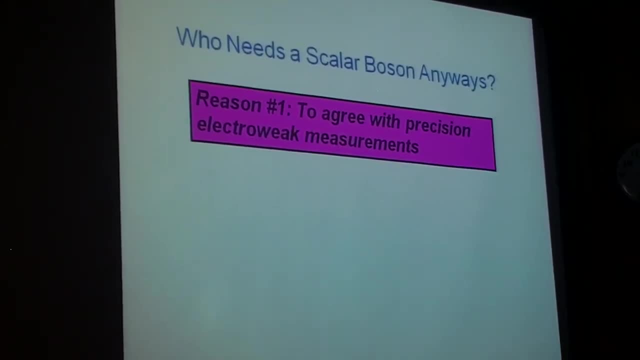 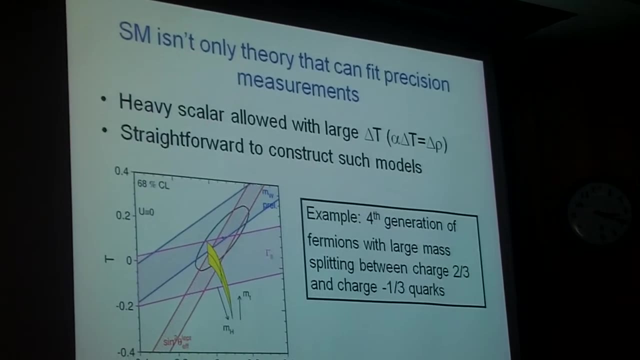 it to agree with all the electroweak precision measurements, because all this data fits this theory perfectly Okay. However, the standard model isn't the only theory that can predict these measurements. It's easy- It's duck soup- to take this model of electroweak symmetry. 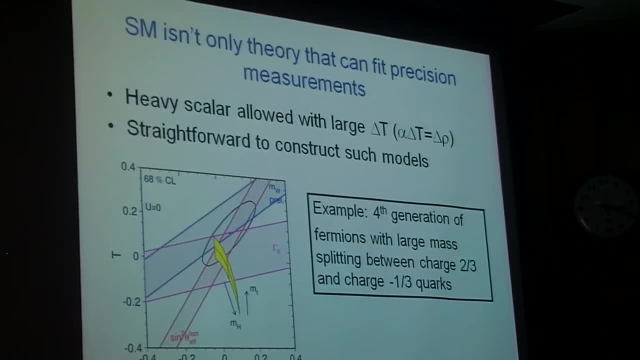 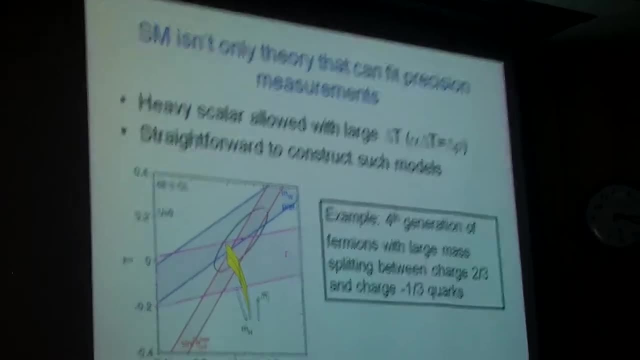 breaking and complicate it and expand it. Thank you. To make it more complicated This particular plot. on this axis is isospin violation And on this axis is essentially the running of the Z propagator from Q squared of 0 up to. 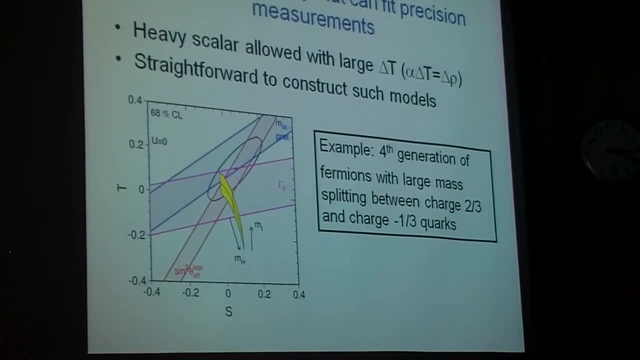 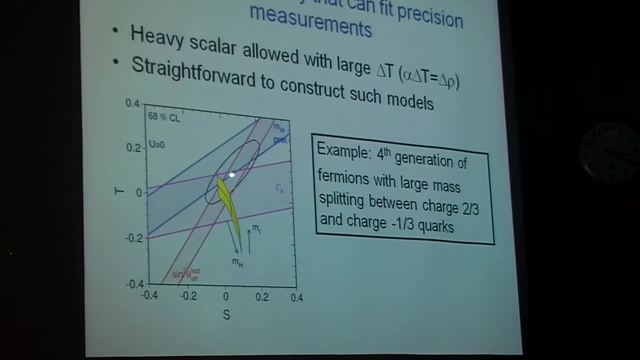 Q squared of MZ squared, And then it fits to the exactly the same data as on the previous slide. So here's the fits to the W mass, for example, And the black dot in the middle is the fit from all this data. And as you try to make the scalar heavier, heavier in this, 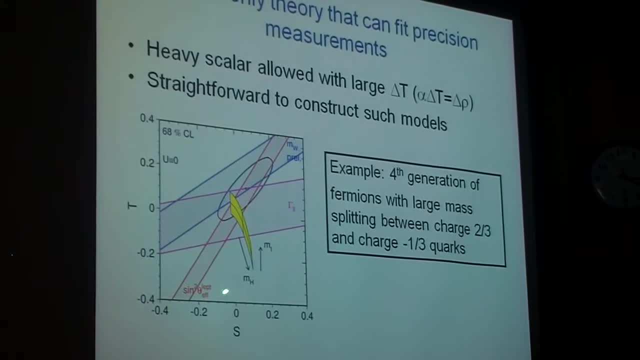 185 GDB. you move away from the Z propagator And then you try to make the scalar heavier from the data. Okay, So it's easy. What do I have to do if I want to have, say, a 1TB? 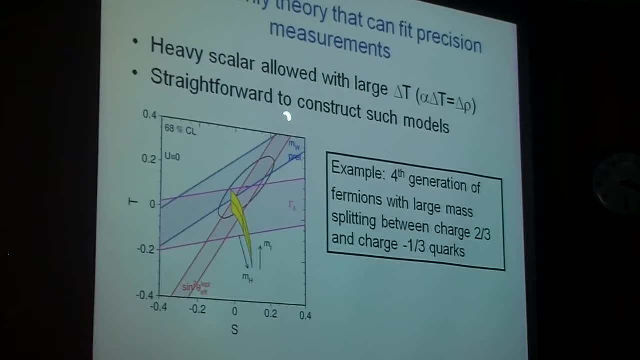 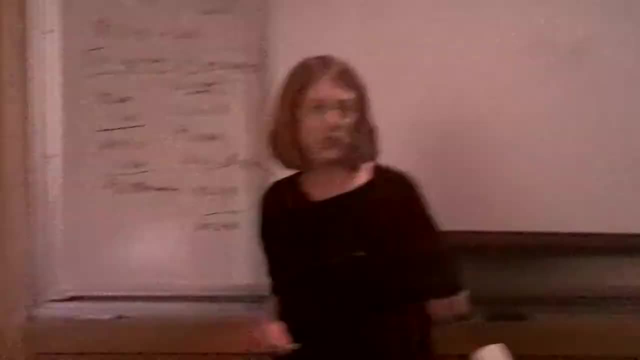 scalar particle, I need to construct a theory with a large positive delta T to get me back up to the fit, And so one example would be a fourth generation of fermions with a large mass splitting. That'll do it. There are lots of ways to do it. So if I have a theory where 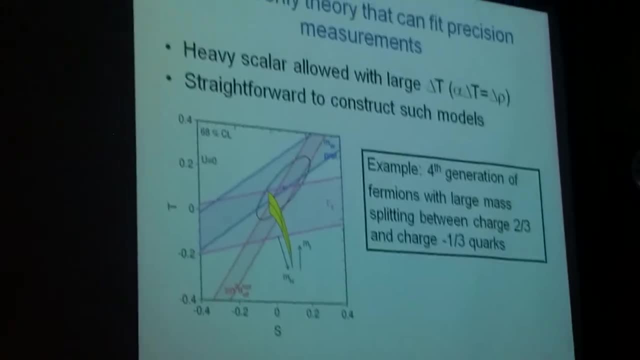 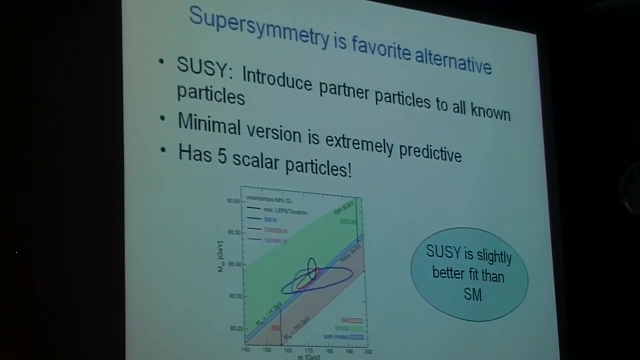 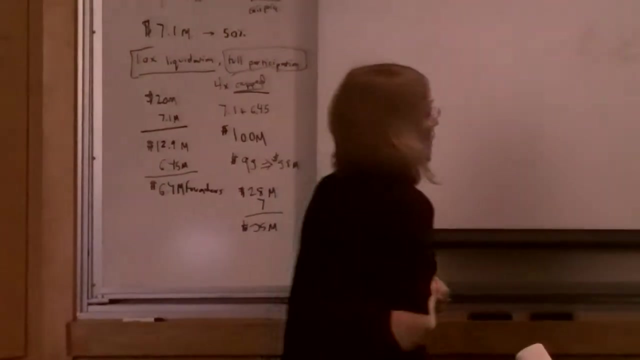 this scalar is heavier than these limits. there's going to be something else which puts me back into agreement with all my data. Okay, Supersymmetry is a favorite alternative to the standard model. If you want to compare your predictions with the predictions of some other theory, well, supersymmetry is our favorite. 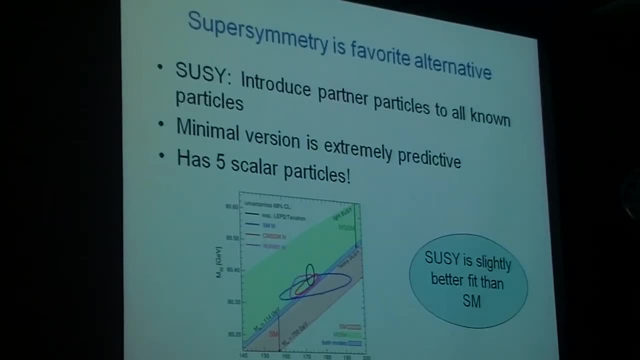 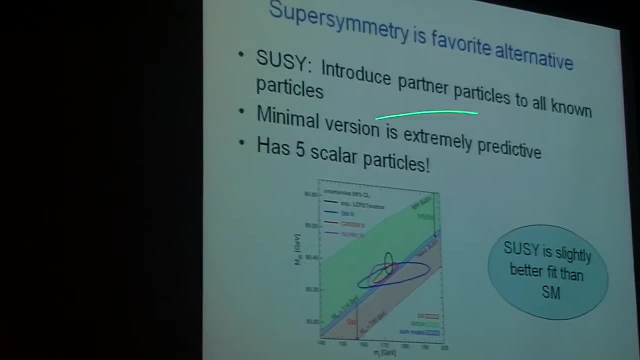 So supersymmetry: you have a partner particle for all the known particles. The electroweak symmetry breaking is broken in exactly the same way as in the standard model, except you have five scalar particles now instead of just one. But the nice thing about supersymmetry: 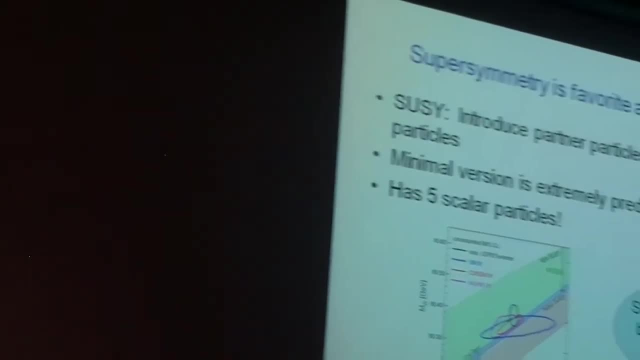 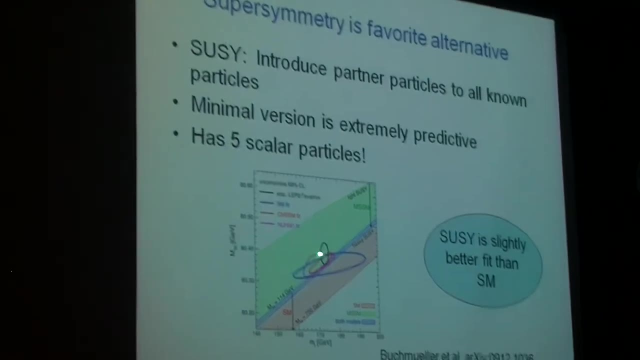 is that the minimal version is extremely predictive. So this is exactly the same thing as the standard model. It's the same plot as I showed you before: the top quark mass and the W mass, The black curve is the experimental numbers and the blue curve is the standard model fit. 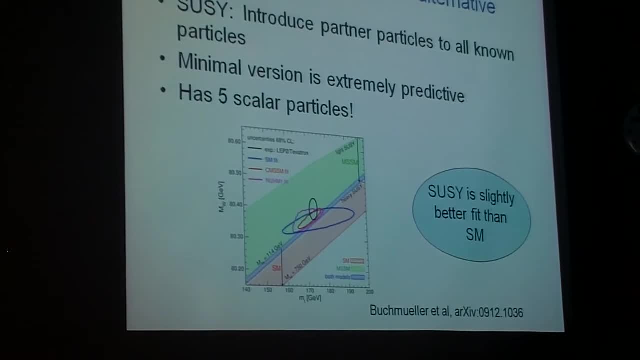 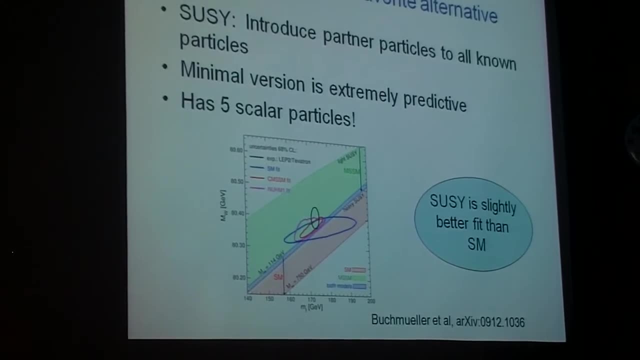 So those are the same curves I showed you before, And in the minimal supersymmetric theory you get this red curve or this pink curve. So the minimal supersymmetric theory with five scalars can fit our data too. In fact, it's a slightly better chi-squared fit. 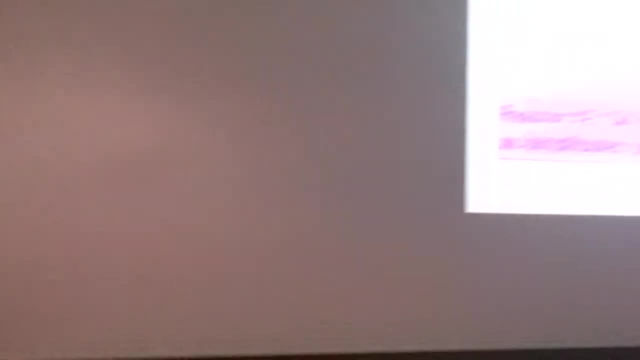 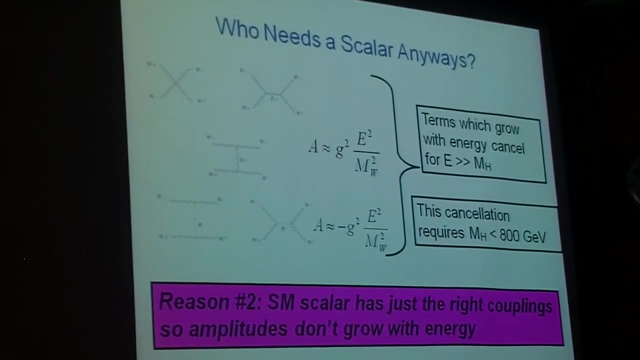 Okay, All right To continue. well, who needs a scalar anyways? Okay, Well, we fit our data with it. but it also has a theoretical reason. If I look at W-W scatter, so W plus, W minus goes to W plus. 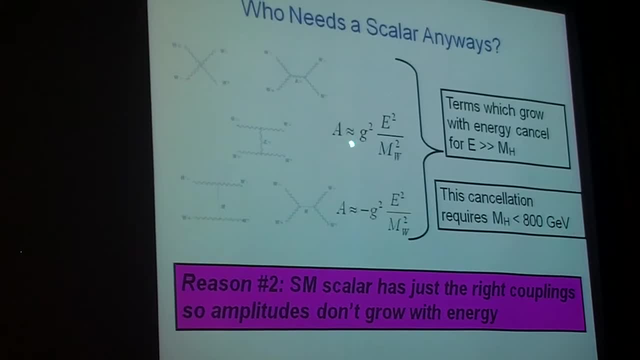 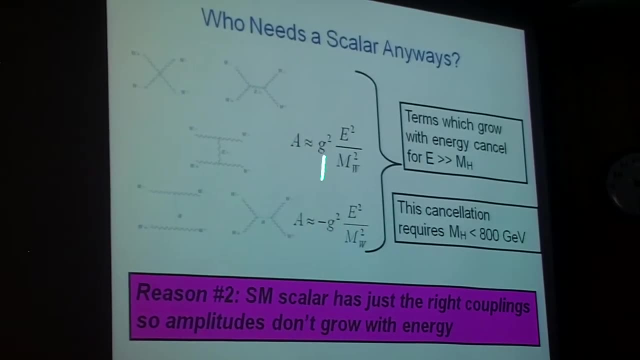 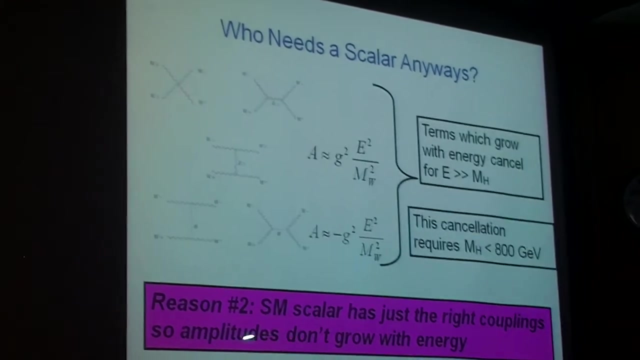 W minus. the amplitudes with gauge boson exchange grow with energy. The amplitudes with scalar exchange also grow with energy. but the couplings are exactly right so that the contributions which grow with energy cancel Okay. So the standard model, scalar, has just the right number. 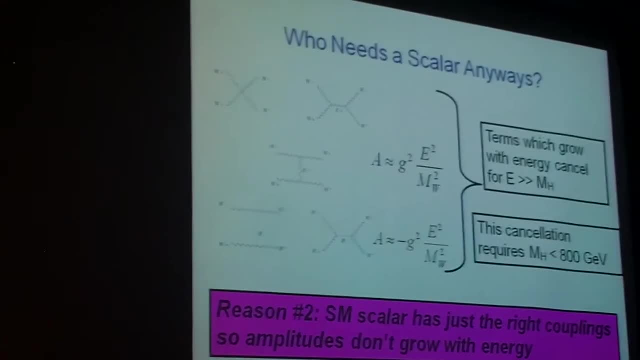 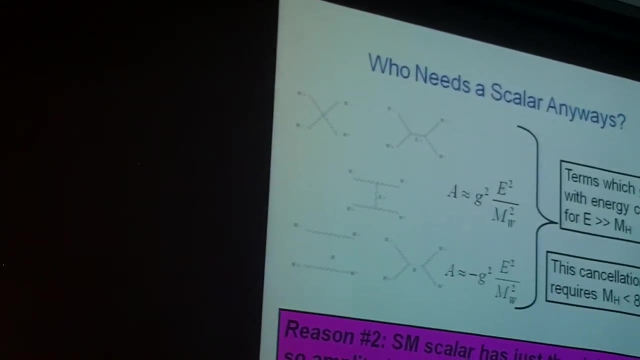 of couplings and the crappy rules are the right couplings so the amplitudes don't grow with energy. So if I start messing around with my theory, adding new particles, new couplings, here, I change this cancellation Okay. So what does this mean? Well, on, very 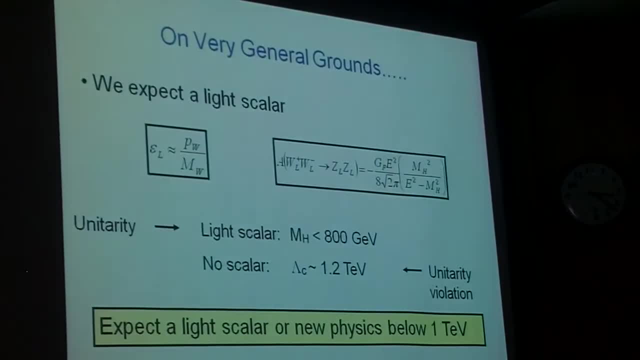 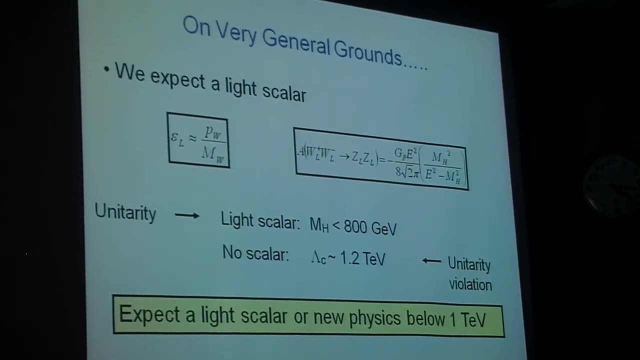 general grounds, we expect that the scalar is relatively light. If I look at the polarization of these W particles, the polarization vector is just their energy over MW. So the scattering of the longitudinal gauge bosons has a piece which grows with energy right and now. if 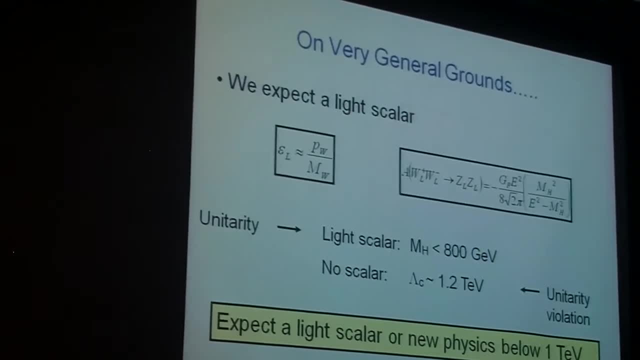 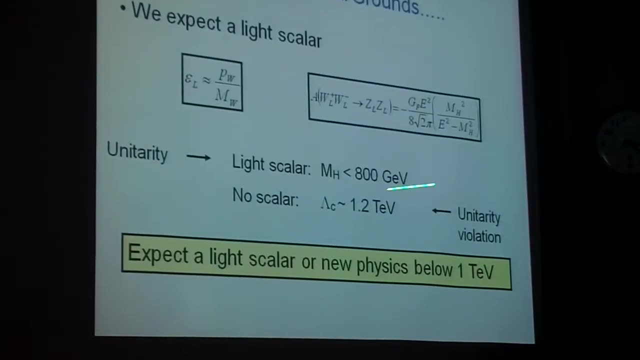 piece which grows with energy and then a piece which is cut off by the scalar mass. So unitarity conservation, the conservation of probability, requires either that the scalar is relatively light, less than about 800 GeV, or if I remove the scalar from the theory. 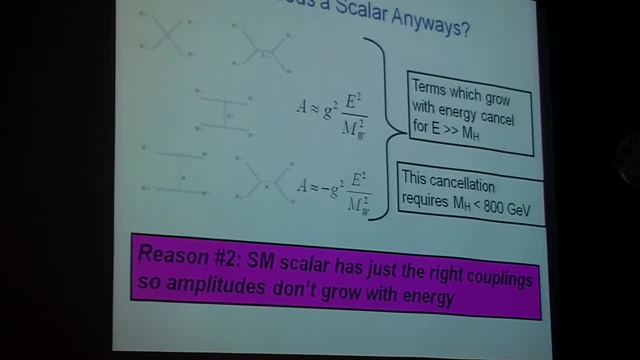 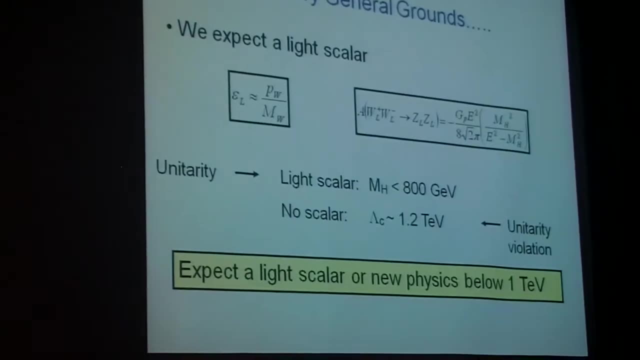 if I go back here and just remove these pieces with the scalar, then something happens at a rounded TeV, and hence my statement that the LHC is the machine we need, Because if I don't see my light scalar, well, then something's going to happen around 1.2. 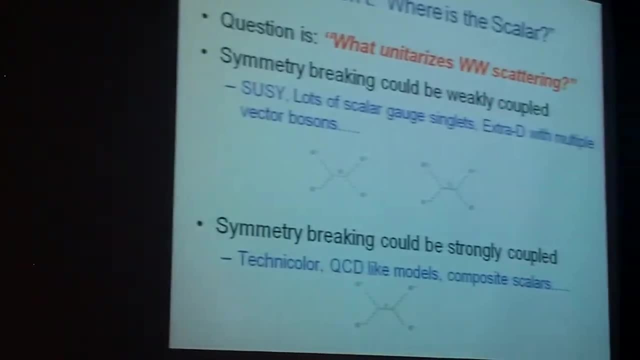 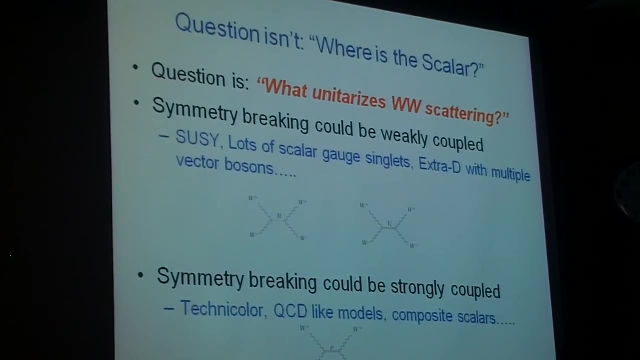 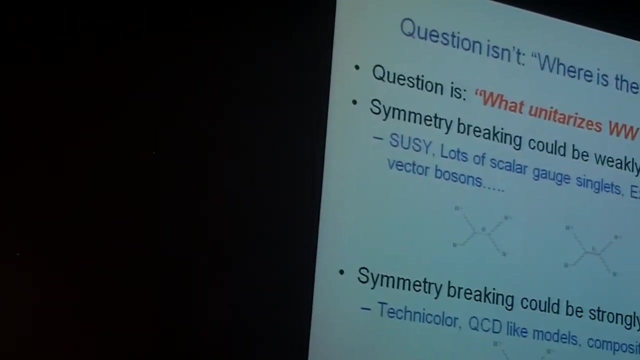 TeV. Okay, So the question really isn't where is the scalar, but rather what unitarizes the W-W scattering. So the symmetry could be weakly coupled. like supersymmetry, where you have lots of things. You can have a lot of scalar gauge singlets here. 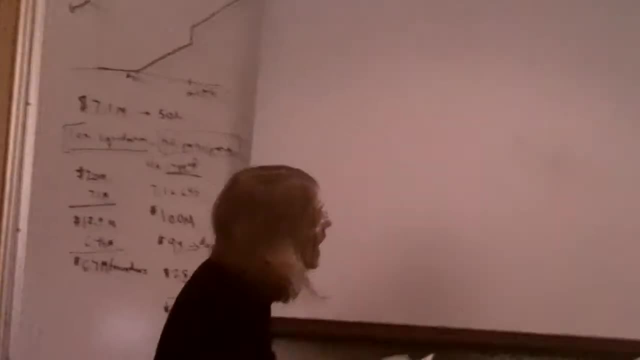 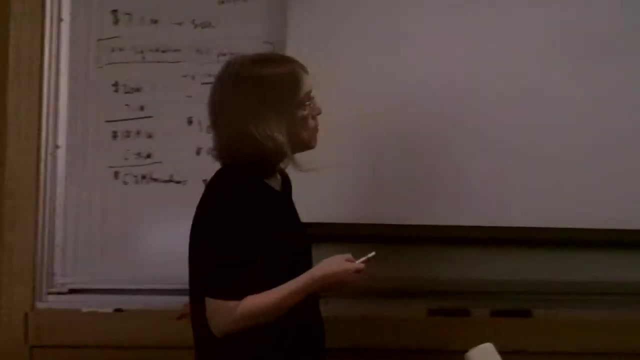 The happy particle could be a series of happy particles, singlets here, And in fact this is particularly nice because the lightest could be a dark matter. You could have extra dimension models with multiple vector bosons which unitarize the theory. 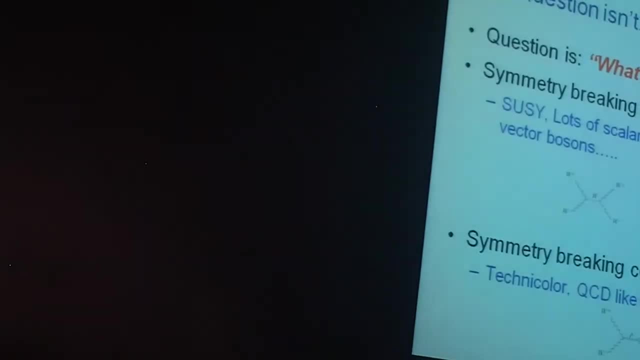 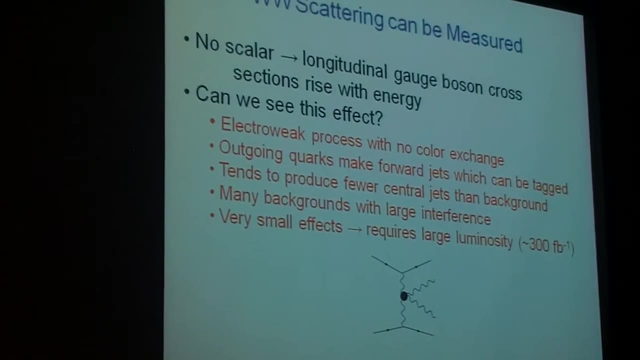 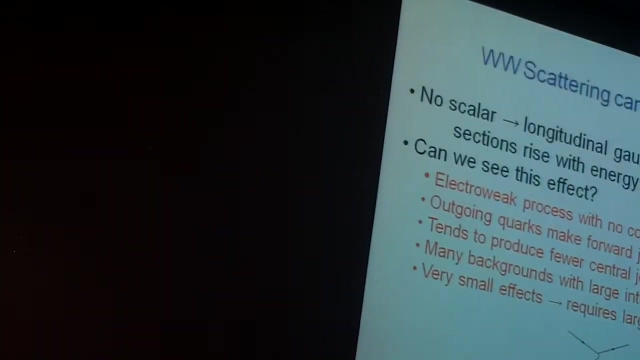 Symmetry breaking could be strongly coupled and it could be something like a technique row here. So there are lots of possibilities here. So can we measure this? Is this just skedonk and W-W scattering? We don't have beams of W And of course the answer is yes, we do have beams of W particles. 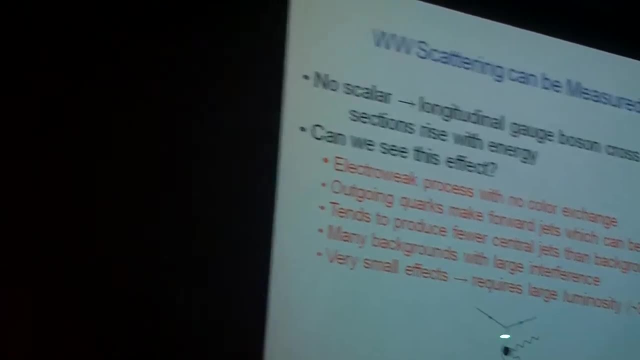 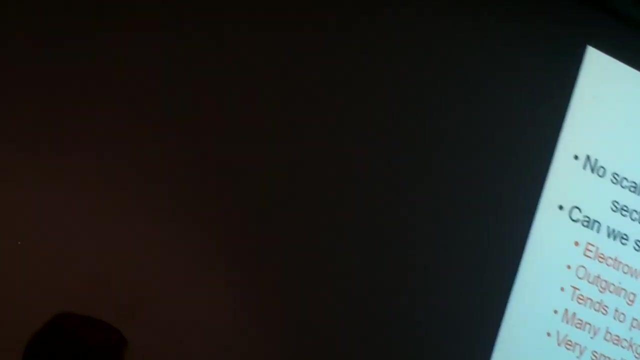 At the LHC. we have quarks here. Here's two quarks Spitting out gauge bosons. this is either a W or a Z interacting to make two gauge bosons coming up. So if we didn't have this scalar, the longitudinal interactions here, gauge boson interactions.